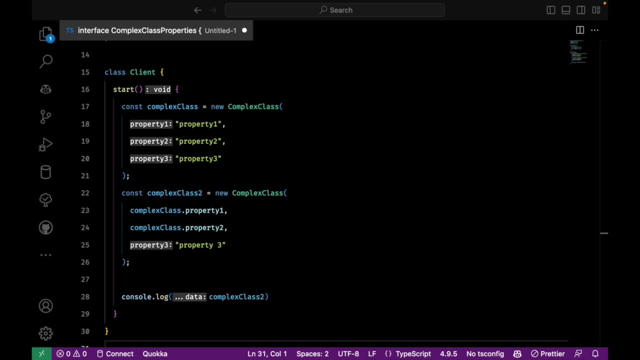 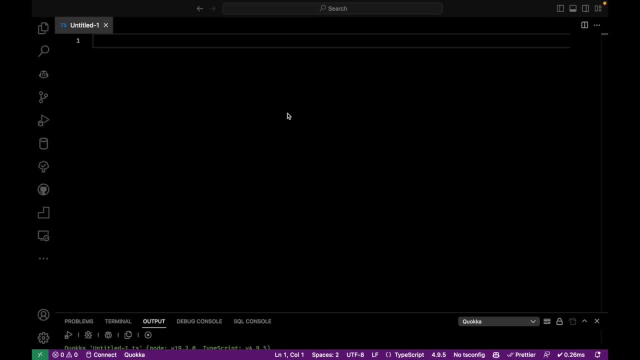 through an interface. You also don't want these concrete classes to be tied coupled to your application. This is what the prototype pattern is for. It lets you create a clone of an existing object instead of creating one from scratch. The first thing you need to do, as always, is to declare your interface. Then you can. 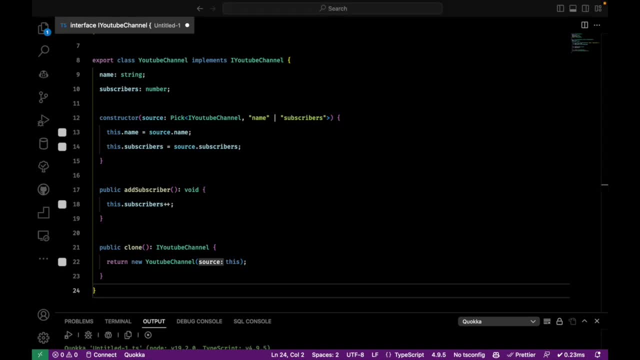 create your prototype class that will implement this interface. In the constructor, you can see that I'm receiving an object that represents the source of information that implements the interface. We also have an actual implementation for the clone method, returning a new instance of the class, and it receives this as argument. The client will be an application that creates. 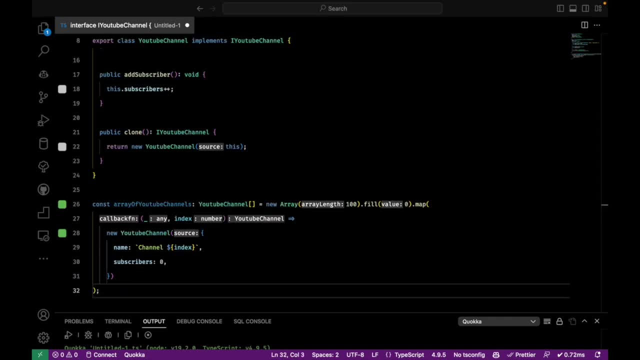 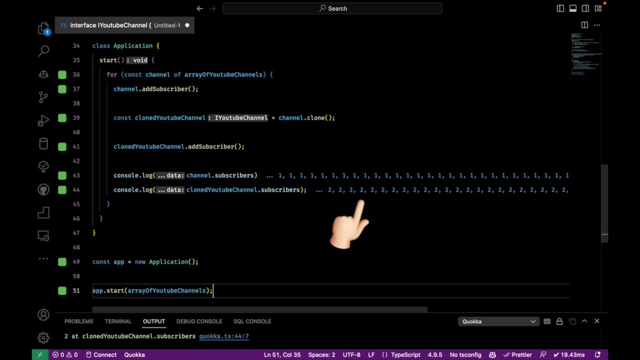 a bunch of YouTube channels but needs to clone them to slightly alter its behavior by adding more subscribers. What you'll see in the logs is that the subscriber counts for the channel and clone's YouTube channel are going to differ by one, because only the 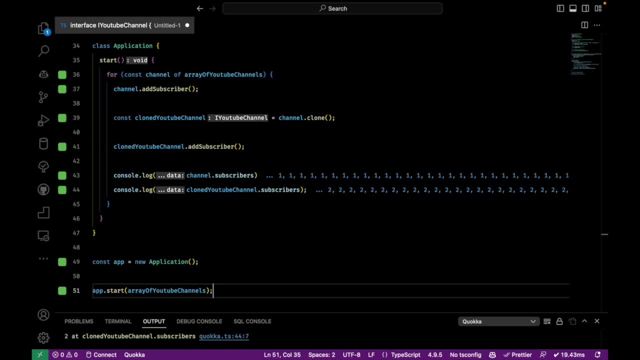 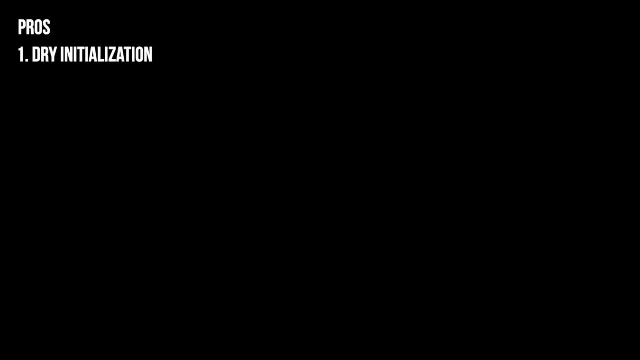 clone method was called, So we can consider this as a new method. The pros for this pattern? First one is that you can get rid of initialization code when you clone pre-built classes. You can produce complex classes more conveniently and it's an alternative to inheritance. 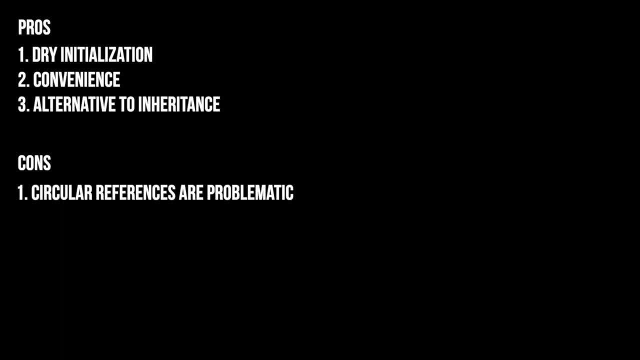 The cons of it is that cloning objects with circular reference just sucks. New projects tend to start using the factory method pattern for creating objects and they end up evolving to use other patterns like the abstract factory pattern. And that's it, folks. This is the simplest I could get with this pattern. 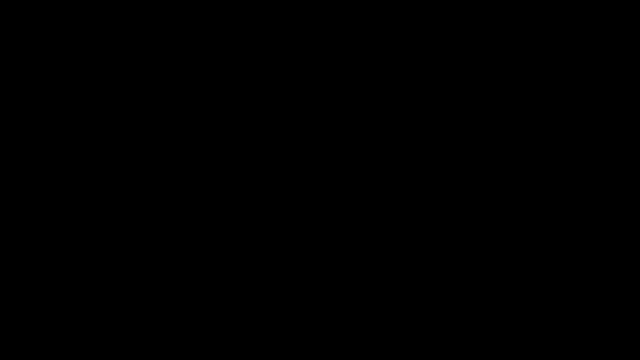 If you enjoyed, don't forget to hit the like, subscribe for more videos and see you in the next one. Bye.